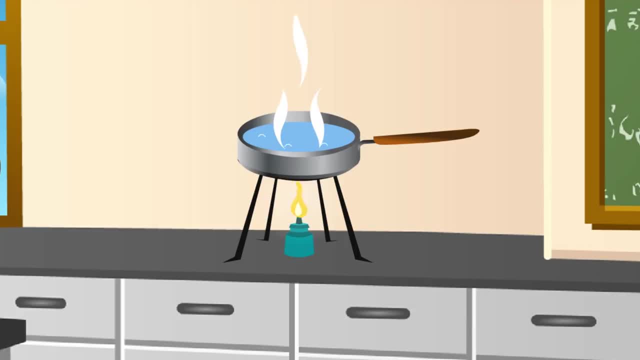 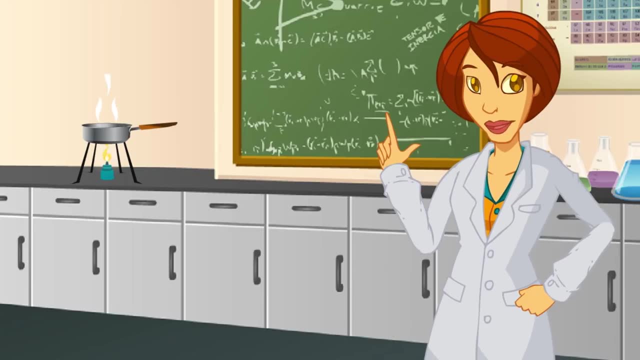 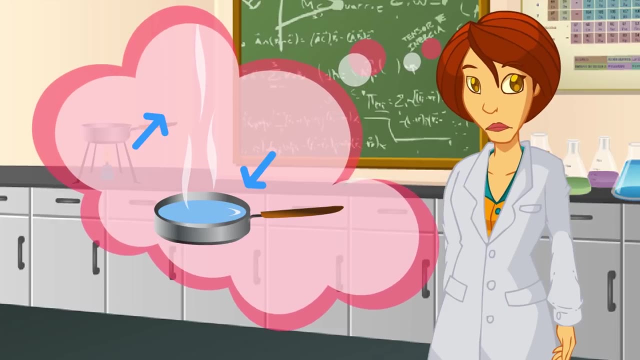 Isn't there anything coming out of the water? Yes, vapor is coming out Because the water is about to boil. Very good, the water has nearly come to the boil. In other words, it has almost reached its boiling point, because we have raised this temperature by means of the fire. Now there's the liquid in the pot and the vapor coming out of it. Which of them is water? The water is in the pot, wasn't it? Yes, very use. Which one is this water? Is it classroom or work? Which Doggy and the Dgg? Which Doggy and the Dgg? Would you recommend us to learn how to put these things together? Do you have any idea? Josh could help out here. Do you have any ideas to beat Christmas answers? Can you talk to your Dgg? 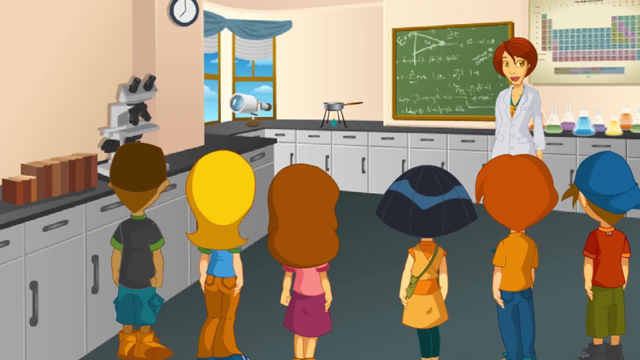 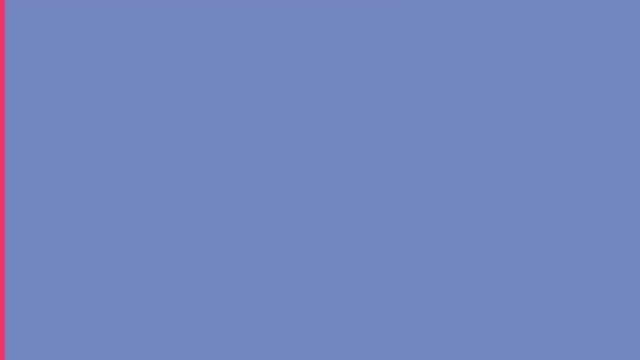 What's coming out of? it is a vapor. No, both are water, but it's in two different states. See, The matter that surrounds us can be found in at least three different states or phases: Solid, liquid and gaseous. 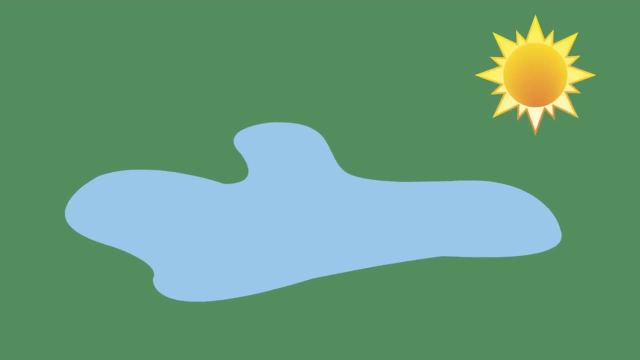 Besides, it can change phases. In this case, water turned from liquid state into gaseous state. This phase transition is called evaporation and occurs on the surface of the liquid. Can we change it again from the gaseous back into the liquid state? 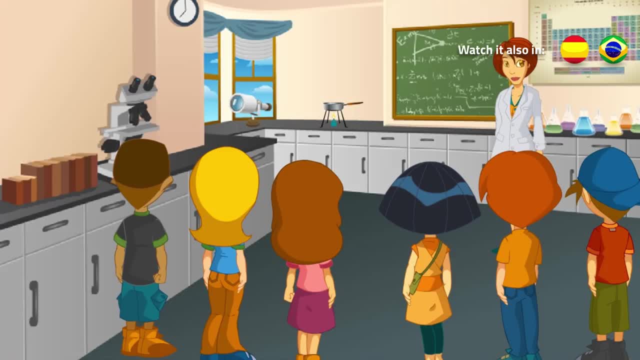 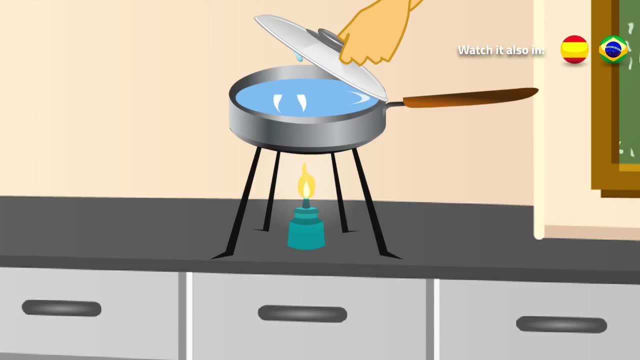 Yes, that's the second part of our experiment. Please see what happens: when I slam the lid on top of the pot, Some drops of water are formed and fall again into the pot. In other words, water vapor returns to the liquid state when it hits the lid and falls. 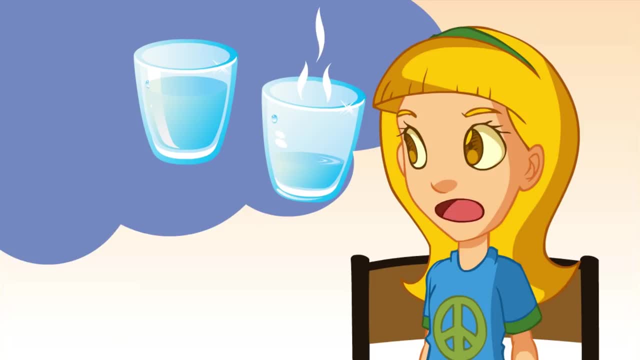 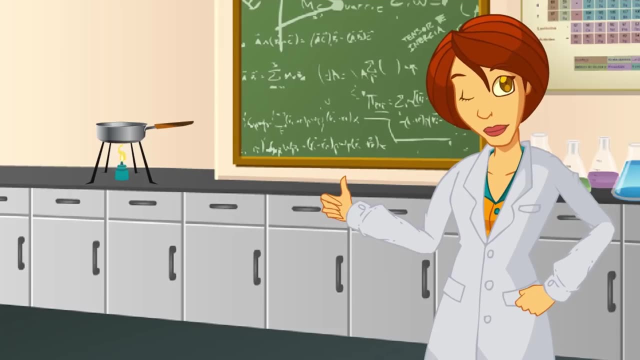 into the pot again. You've said that matter has three states. We've already mentioned the gaseous and the liquid. There's still one missing: the solid state. Excellent, What's the solid state of the water? Ice Right. 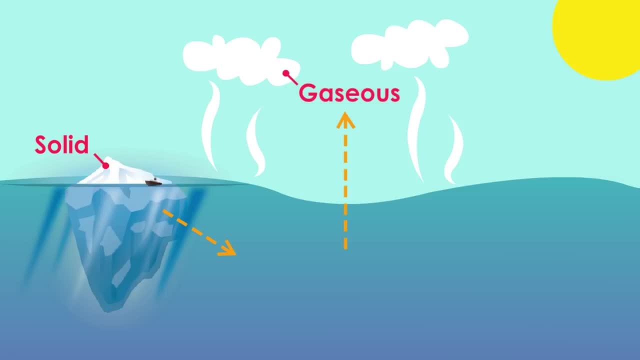 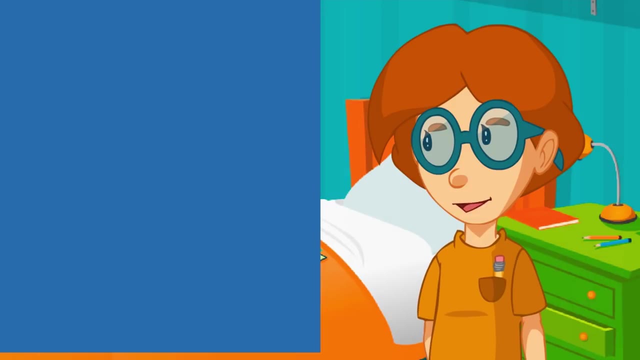 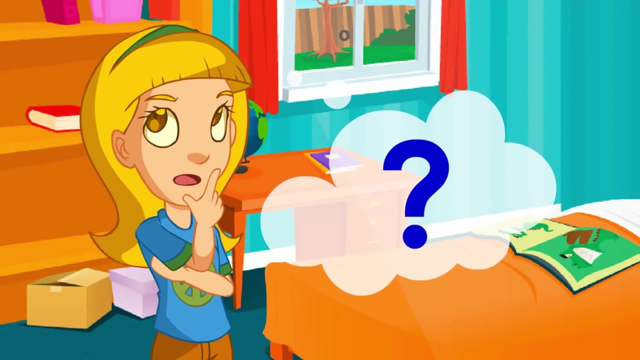 I've made a diagram on the blackboard for you to see how water changes from one phase into another. I know what happened to the mothballs: They change from a ball-solid state into a smelling gaseous state. A ball-solid state into a smelling gaseous state. 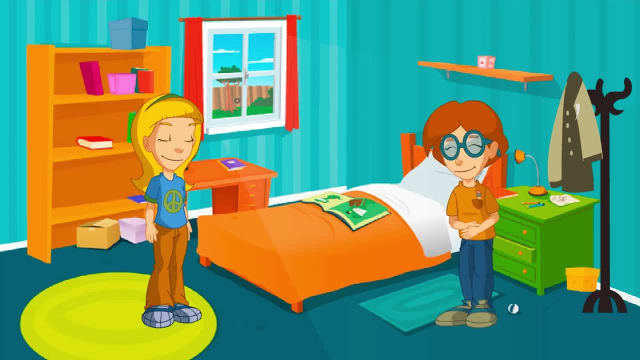 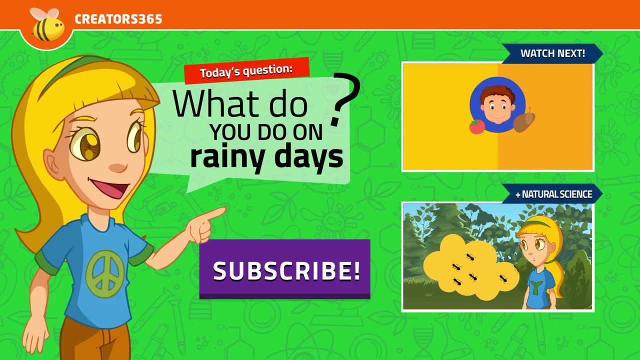 What's that? It's simple Nat Moth poison. Hey, don't forget to subscribe and answer the questions. See you next time, Bye, Bye, Bye, Bye. You can also click the links on the right to continue learning and click the Like button. We appreciate your help, See ya.